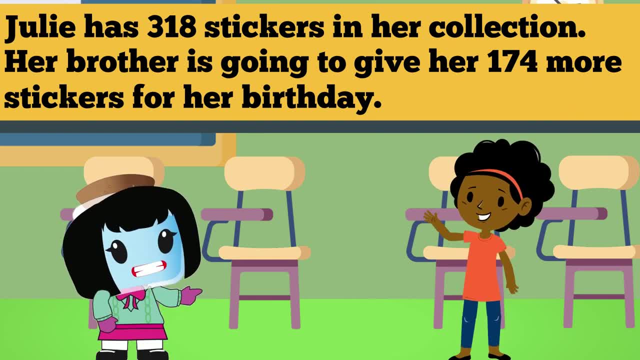 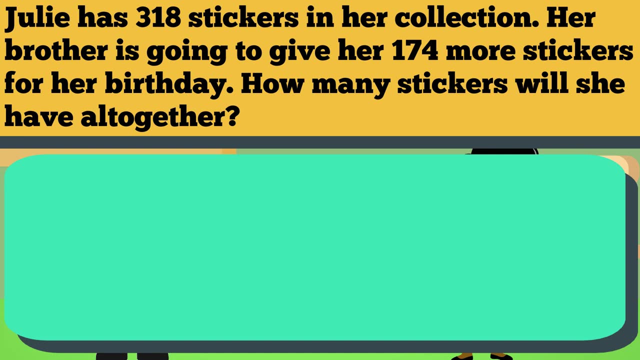 Julie has 318 stickers in her collection. Her brother is going to give her 174 more stickers for her birthday. How many stickers will she have altogether? So we know what Julie has- 318, and we know what her brother is going to give her- 174.. 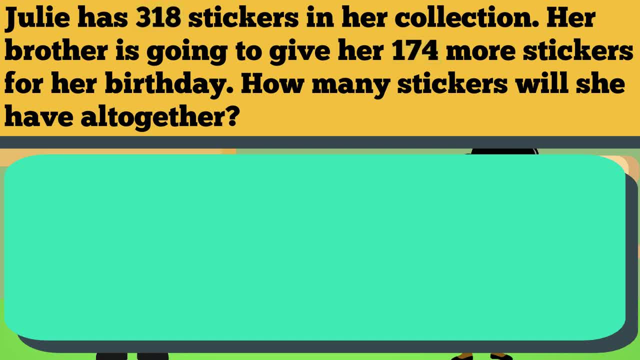 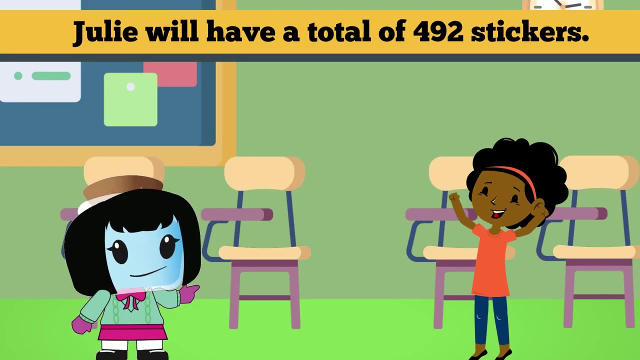 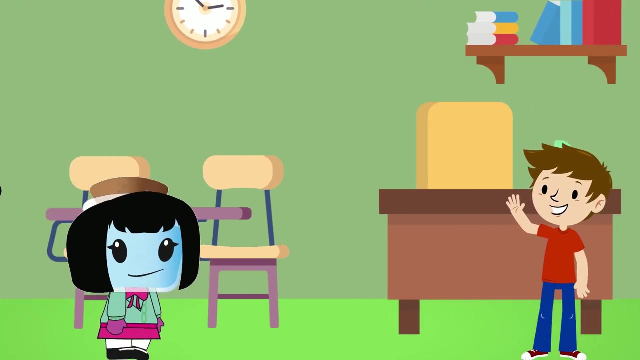 How do we figure out the total amount of stickers that she'll have? Yes, we need to add 318 plus 174.. what did you get? 492 is correct. Julie will have a total of 492 stickers. do you mind helping with one last problem? 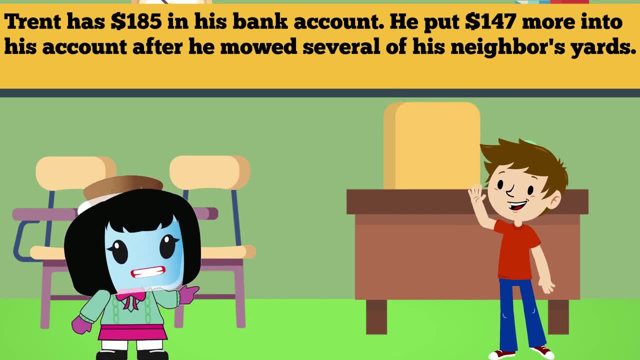 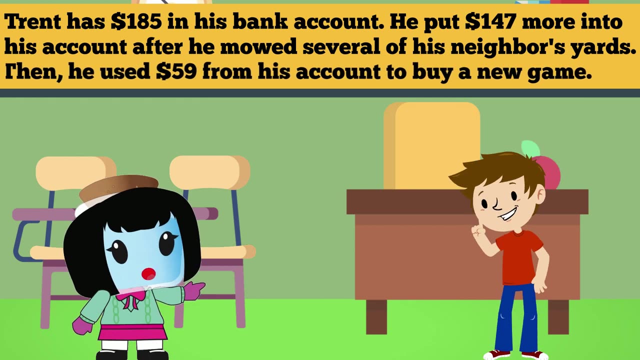 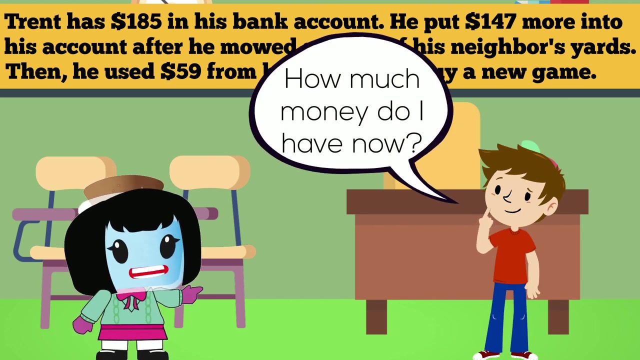 Trent has $185 in his bank account. he put a hundred and forty seven dollars more into his account after he moved several of his neighbors yards. then he used fifty nine dollars from his account to buy a new game. how much money does he have now? wow, that is a lot of information. 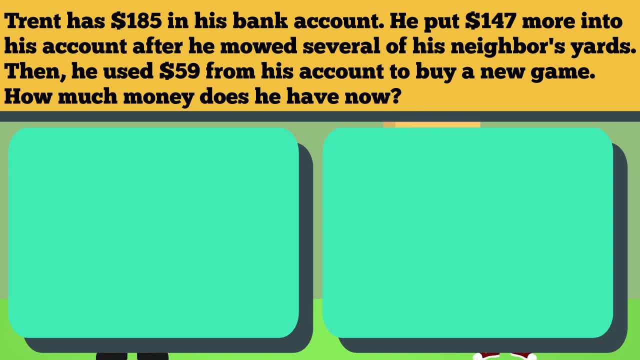 let's look at this one part at a time. we know that he started with $185 and put a hundred forty seven more in. how would we figure out how much? that is great job. we need to add the amounts together: one hundred eighty five plus one hundred forty seven. each of those is $185 and put a hundred forty seven more in. 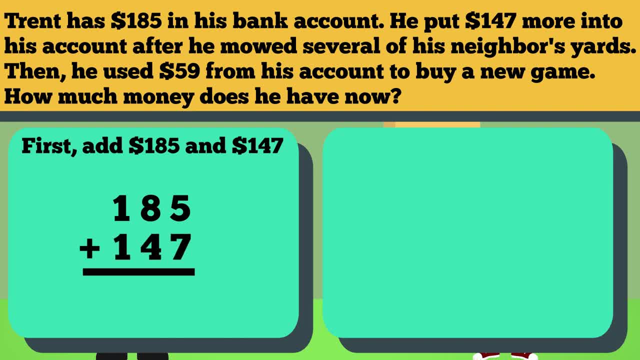 how would we figure out how much that is? great job. we need to add the amounts. sixty four plus four equals three hundred thirty two US dollars in each foarte two. but don't forget he also spent fifty nine dollars on a new game yesterday. wasn't in the land, um, mmhm. 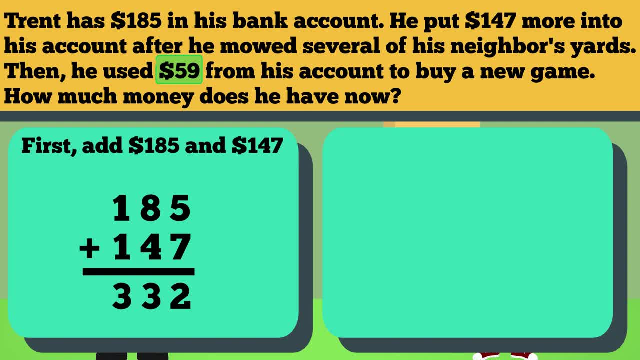 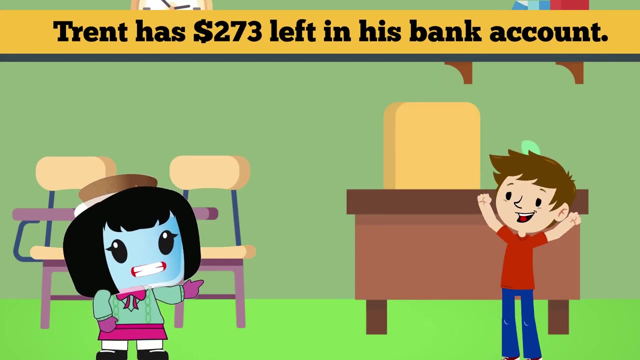 59 on a new game. since he spent that money, we need to subtract it from what he had: three yogurt, three for 34 naturals. text recognition: 34аж thirty-two minus fifty-nine equals 36, Дж equals 273.. So he has $273 left in his bank account. 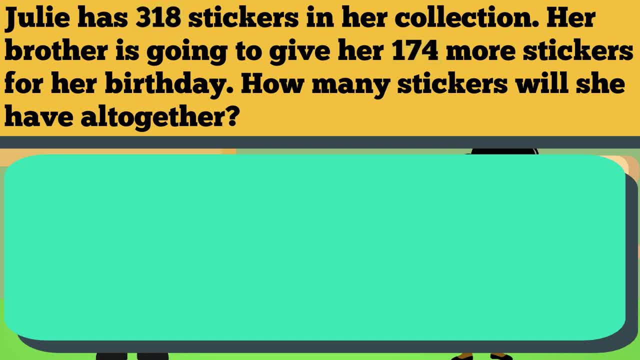 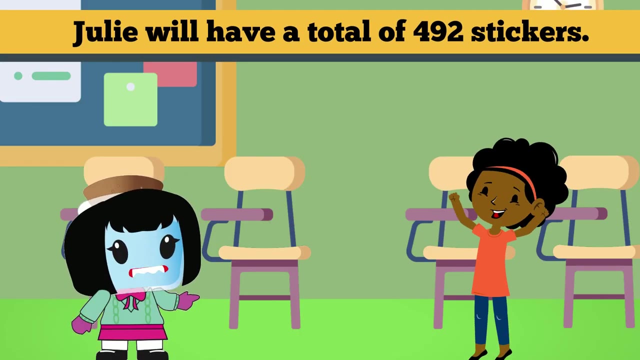 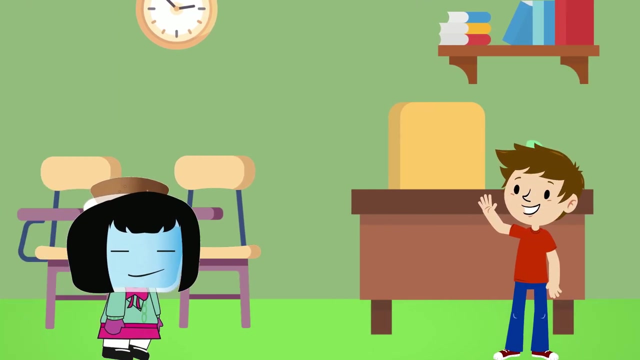 How will we figure out the total amount of stickers that she'll have? Yes, we need to add 318 plus 174.. what did you get? 492 is correct. Julie will have a total of 492 stickers. do you mind helping with one last problem? 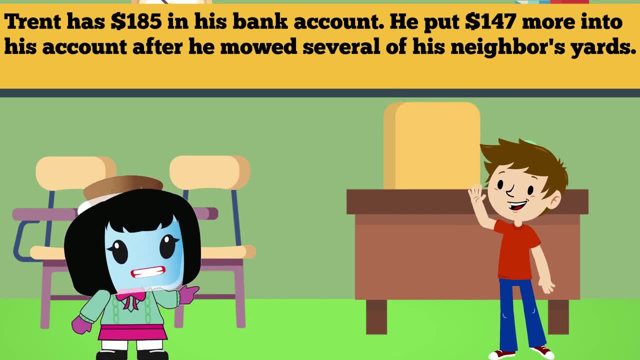 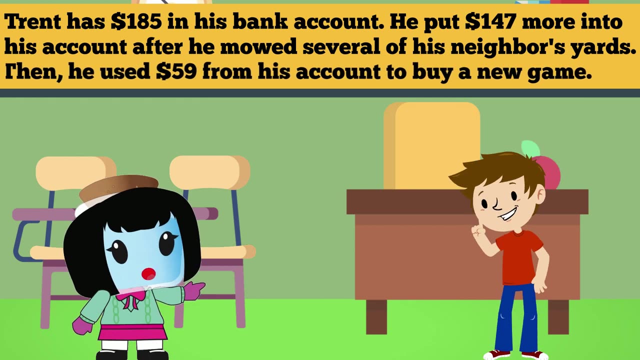 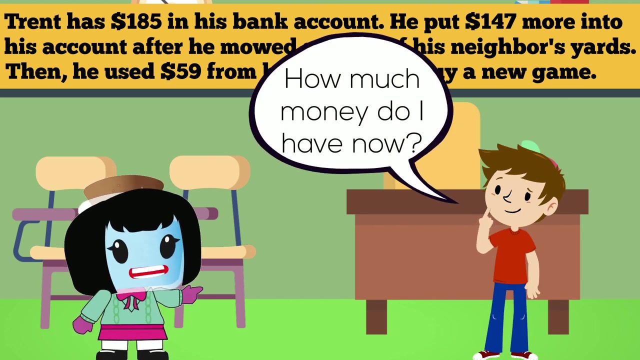 Trent has $185 in his bank account. he put a hundred and forty seven dollars more into his account after he moved several of his neighbors yards. then he used fifty nine dollars from his account to buy a new game. how much money does he have now? wow, that is a lot of information. 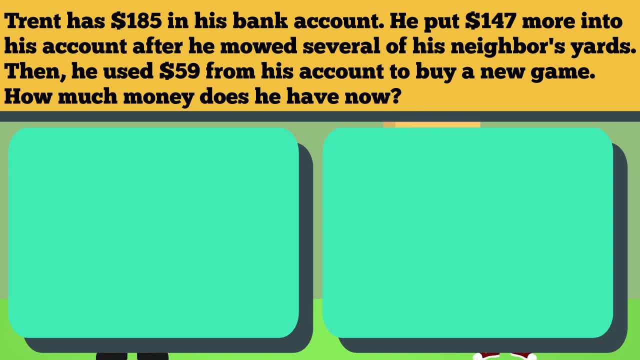 let's look at this one part at a time. we know that he started with $185 and put a hundred forty seven more in. how would we figure out how much? that is great job. we need to add the amounts together: one hundred eighty five plus one hundred forty seven. each of those is $185 and put a hundred forty seven more in. 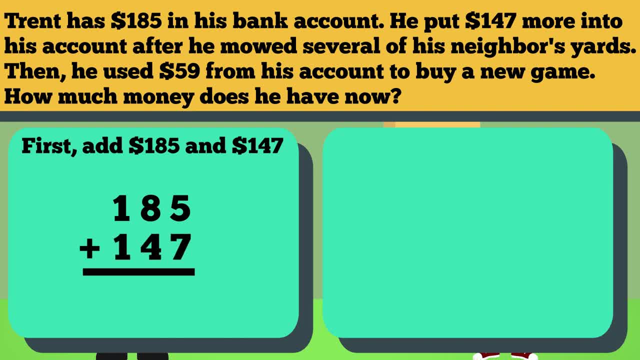 how would we figure out how much? that is great job. we need to add the amounts to that part at a time. we know that he spent someない. I have got a hundred and thirty-two, when another $59 spent on was, so there was no more money on the game and perfect. so here we go again先生, thank you. 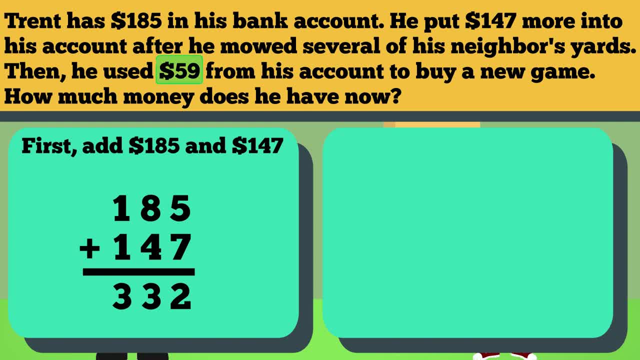 also spent $55 on a new game and he had a hundred and fifty nine dollars in your account. since he had spent the money in every game. he had paid you $ handled, since you spent several羽 over a hundred six hundred thirty five dollars and keep this costs you거야.